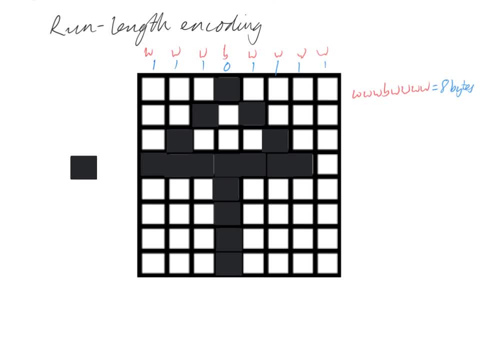 assign a numbered value to it. so, for example, rather than writing out w, w, w, w, so the three w's to start with, we would write three w, okay. then we've got a b next to symbolize um, the black part of the image, so we would write one b. and then we've got four w's. to finish off, just here. 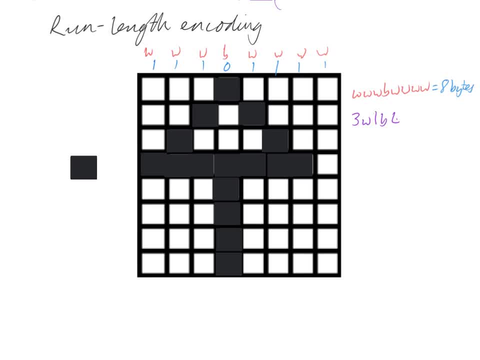 okay, so we would write four w. so if we were then to tally all of this up, in terms of how much space this would take up, um, we can count each byte: one, two, three, four, five, six. so rather than taking up eight bytes, we reduced it to three bytes. so if we were then to tally all of this up, we reduced it. 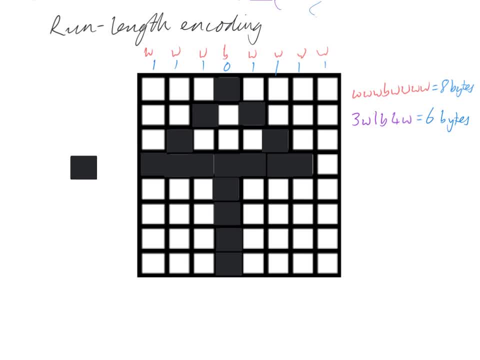 to six bytes. okay, and this is essentially how run length encoding works. it substitutes a sort of string of letters which are the same for a number, signifying the amount of times that letter's there and the letter after it. okay, so our line in this code would be eight bytes if it wasn't run length. 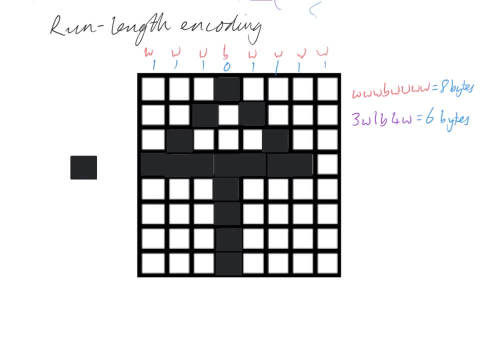 encoded. instead it's six bytes. bytes. if we then kind of extrapolated this outwards for the whole image. we know we've got um eight rows: one, two, three, four, five, six, seven, eight. we know that if we use runtime encoding each row will be six bytes, as we've worked out here. so we can say: 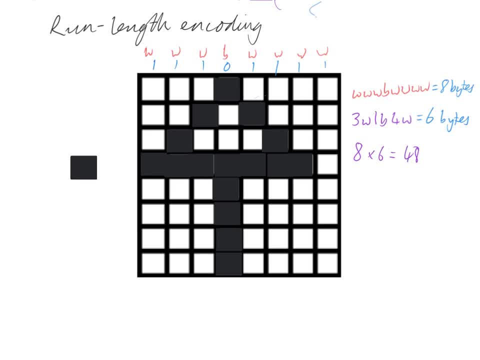 eight times six, which gives us 48 bytes. okay, so if the entire image was run length encoded, that would be how big it is. if it wasn't run length encoded, we'd be looking at eight times eight, which is 64 bytes. okay, so you can see the difference in size there by run length encoding this one image.